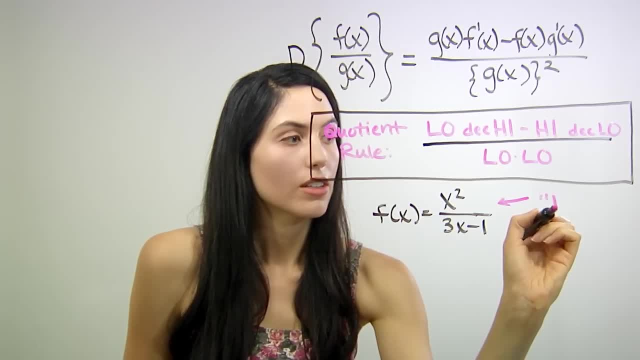 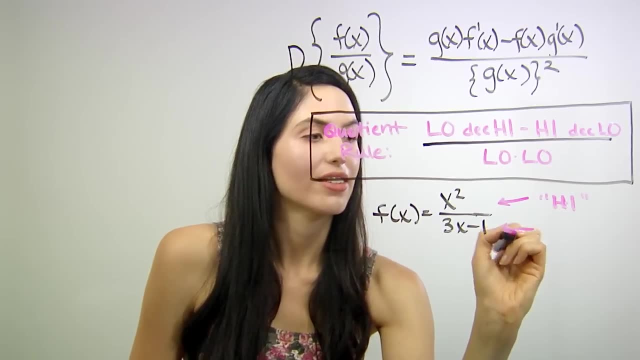 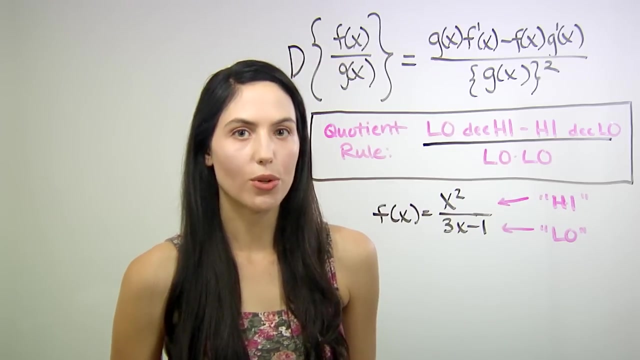 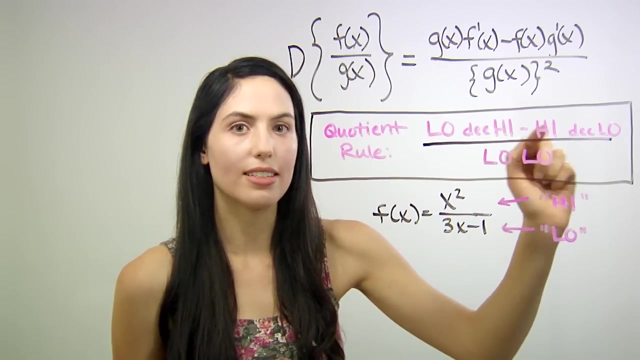 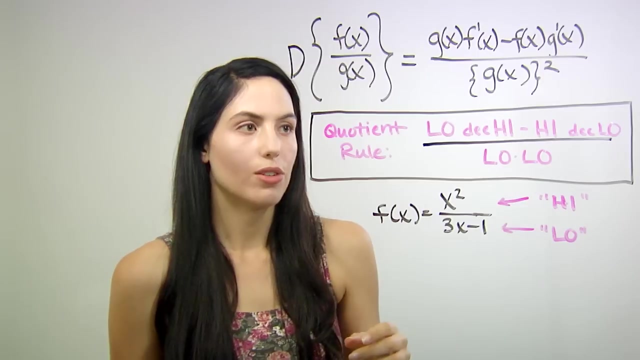 Let's call the top function your high function, and the bottom function the low function. Alright, so here's the shortcut. You can remember the quotient rule by just remembering low d, high minus high d, low over low. low d just means the derivative of. So we have: 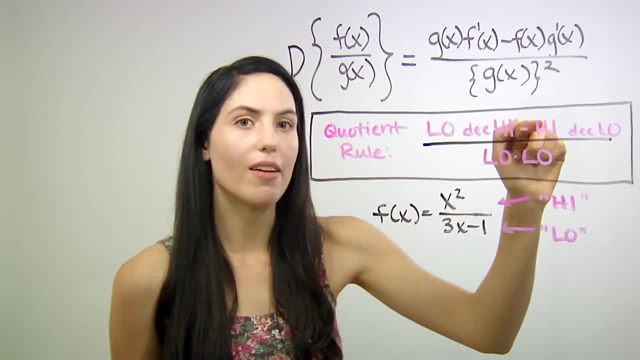 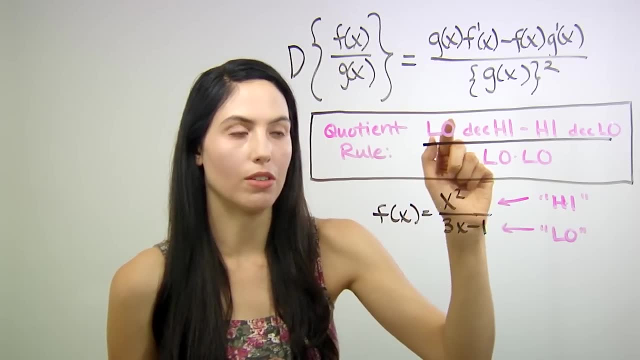 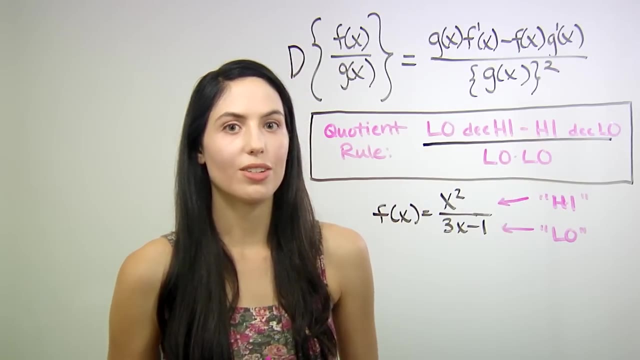 low function times. derivative of high function, minus high function times. derivative of low function, all over low function times. low function, That's just bottom times derivative of top times, top times, derivative of bottom, all over bottom times, bottom. So the shortcut to remember is just low d high, minus high d, low over low, low. 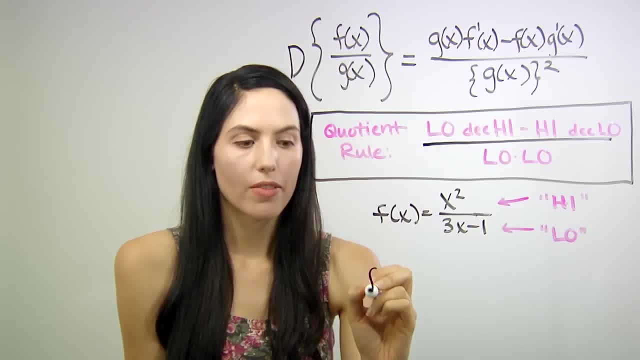 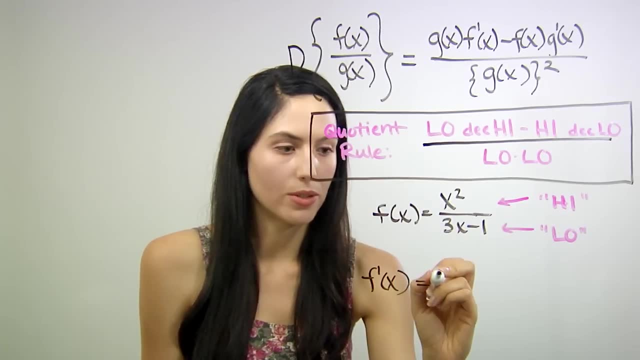 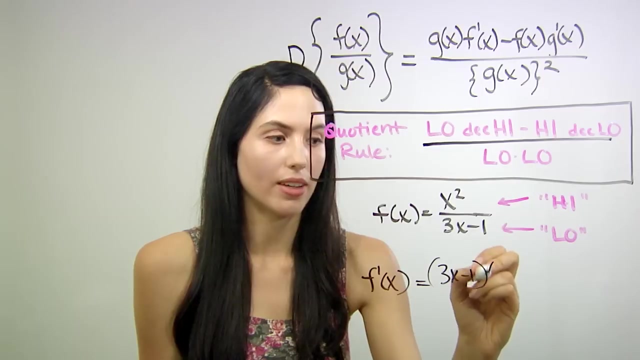 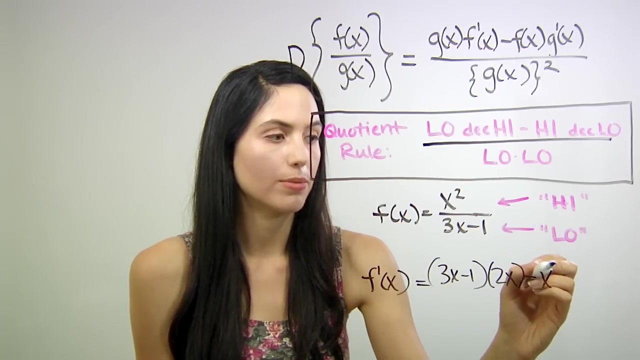 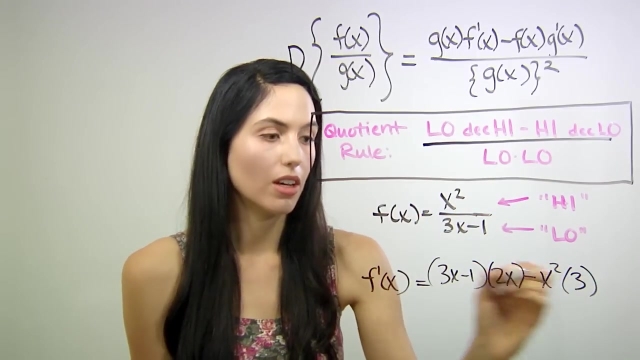 So let's try it. Our function derivative f, prime of x will equal low three x minus one times d high. derivative of x squared two x minus high, just x squared function times d low. derivative of three x minus one, which is three all divided by low low. 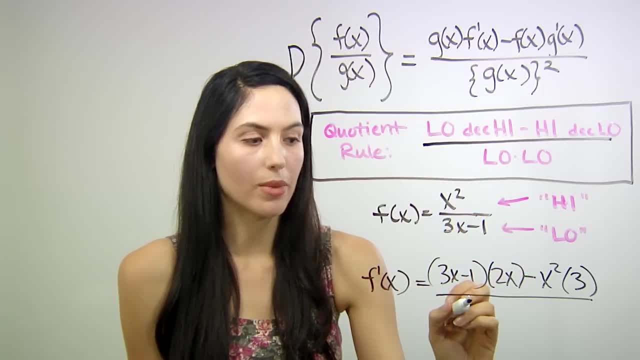 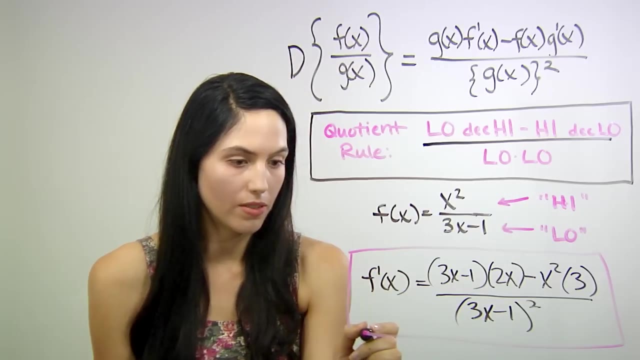 just your bottom function times itself three x minus one, times three x minus one, which can also be written as three x minus one, squared Alright. so that is the answer to the built-in function derivative of our function And that is the answer to your function derivative. 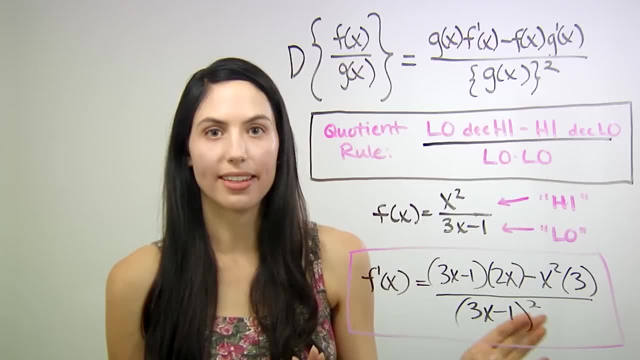 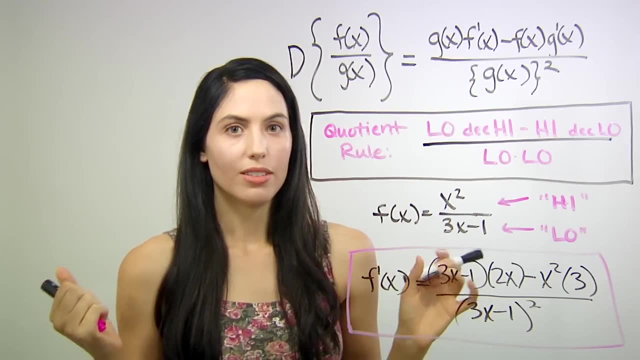 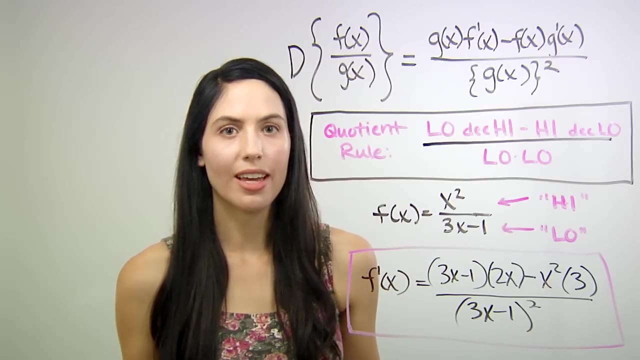 Of course you would need to simplify this answer. You can simplify the numerator, the top, but this is basically it. So you can either remember this or you can just remember low d, high, minus, high d, low over, low, low. kind of dumb when you say it in your head, but it is super helpful. So I hope. 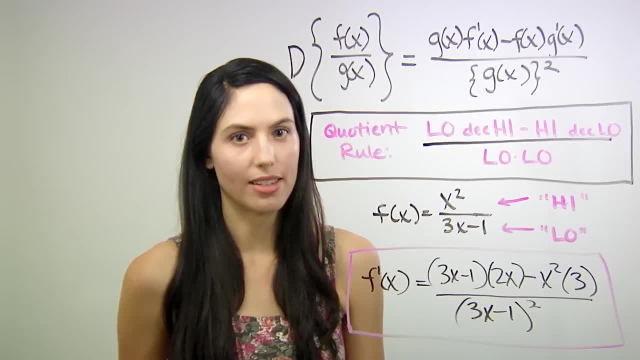 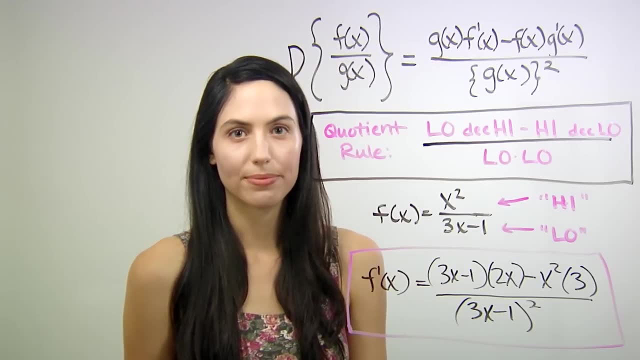 this trick helps Look. anything that makes calculus easier is a good thing, So if you found this helpful, please click like on my video below or subscribe.